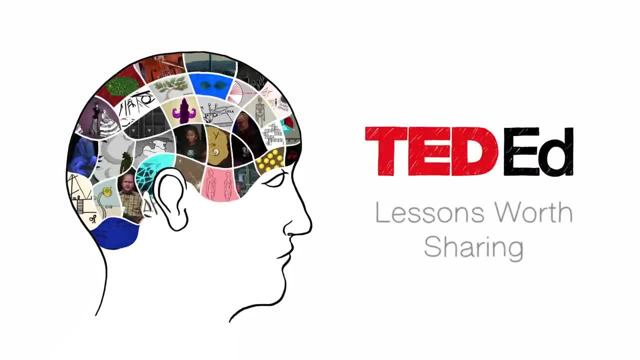 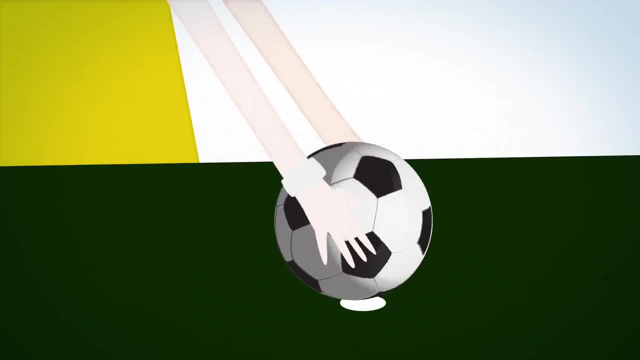 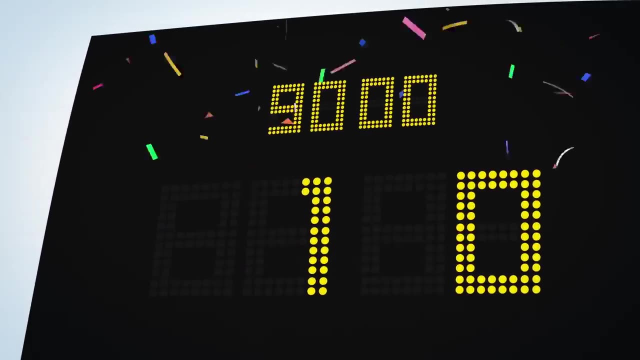 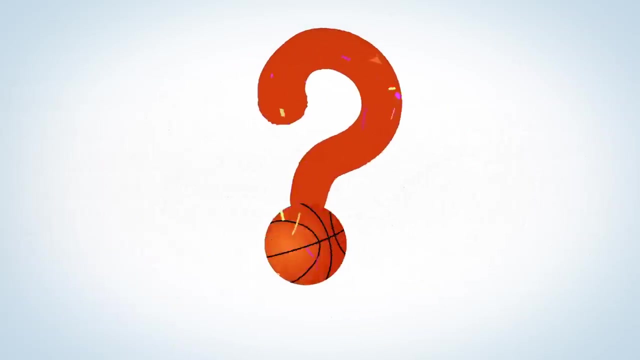 The victory of the underdog over the favored team, The last-minute penalty shot that wins the tournament, The high-energy training montages. Many people love to glorify victory on the playing field, cheer for favorite teams and play sports. But here's a question: Should we be so obsessed with sports? Is 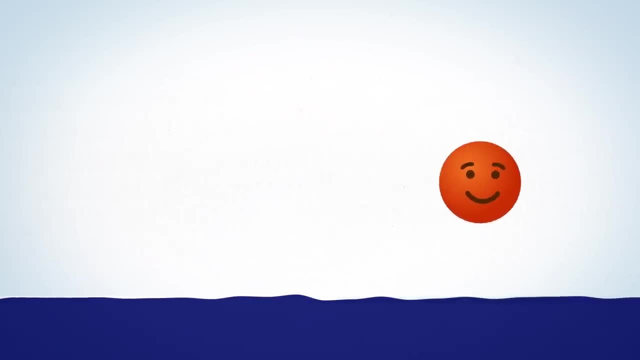 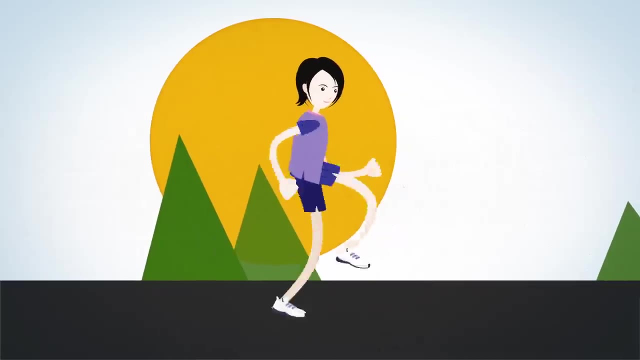 playing sports actually as good for us as we make it out to be, or just a fun and entertaining pastime. What does science have to say? First of all, it's well accepted that exercise is good for our bodies and minds, and that's. 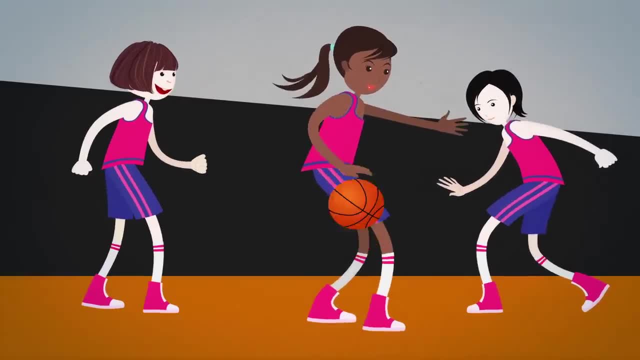 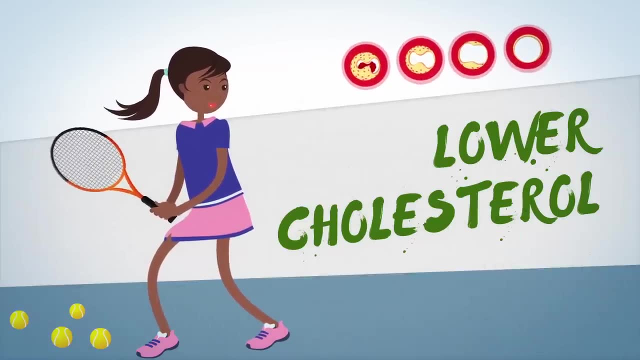 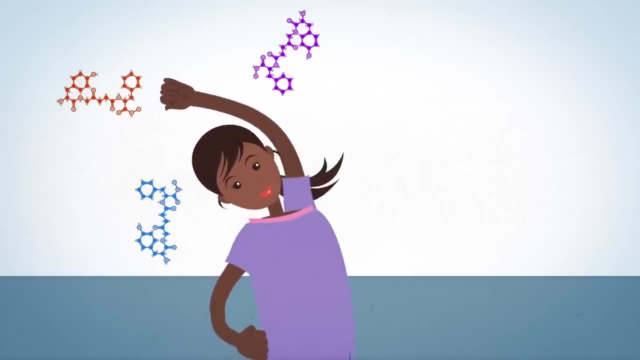 definitely true. Exercising, especially when we're young, has all sorts of health benefits, like strengthening our bones, clearing out bad cholesterol from our arteries and decreasing the risk of stroke, high blood pressure and diabetes. Our brains also release a number of chemicals when we work out, including 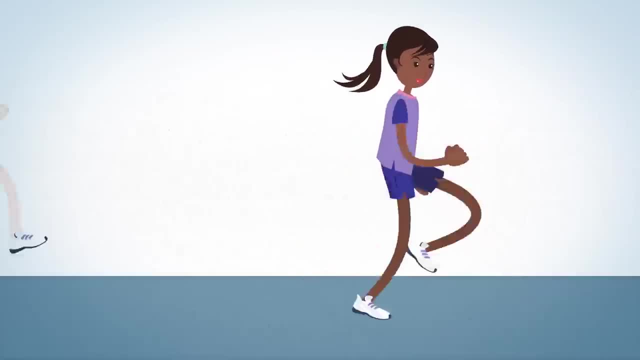 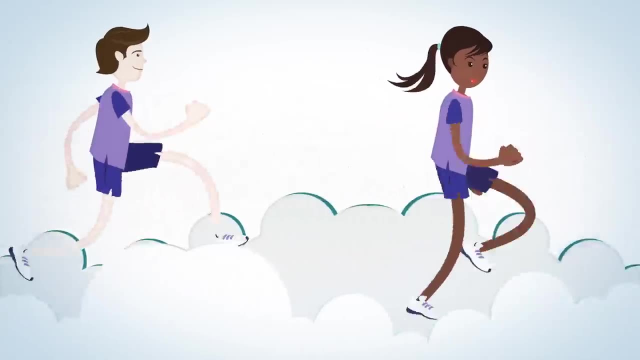 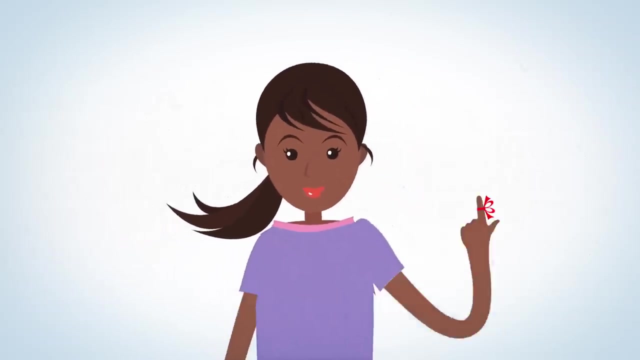 endorphins. These natural hormones, which control pain and pleasure responses in the central nervous system, can lead to feelings of euphoria, or what's often called a runner's high. Increased endorphins and consistent physical activity in general can sharpen your focus and improve your mood and memory. 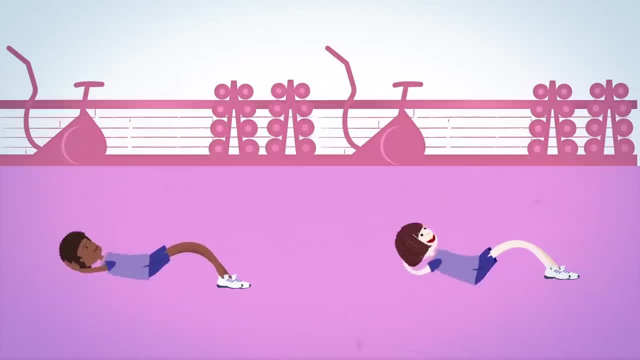 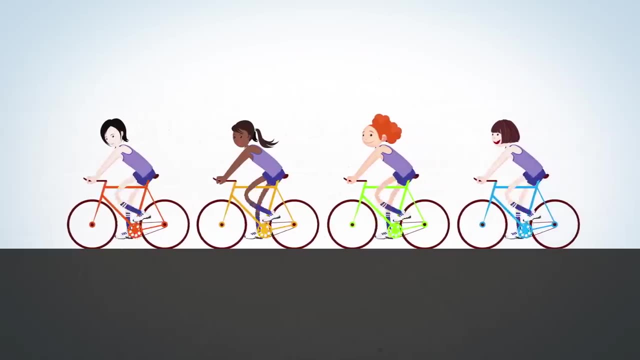 So does that mean we'd get just as much benefit going to the gym five days a week as we would joining a team and competing? Well, here's where it gets interesting, Because it turns out that if you can find a sport and a team you like, studies show that there are all sorts of 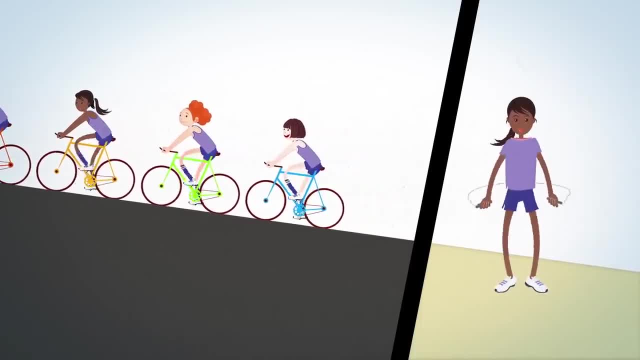 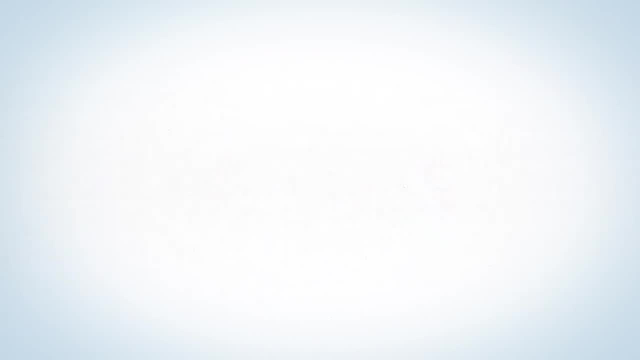 benefits that go beyond the physical and mental benefits of exercise alone. Some of the most significant are psychological benefits, both in the short and long term. Some of those come from the communal experience of being on a team, For instance, learning to trust and depend on others, to accept help, to give. 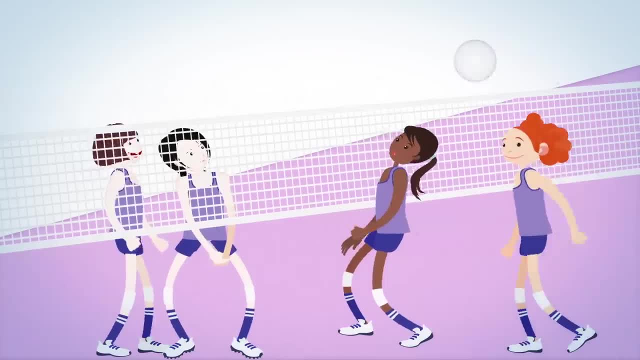 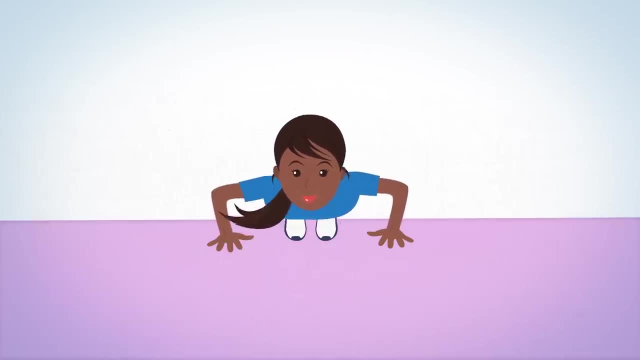 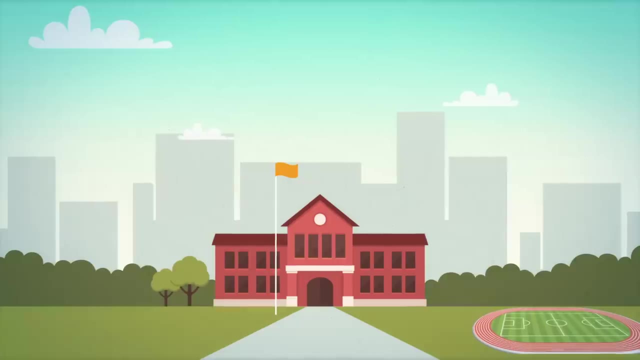 help and to work together to improve our lives. That's the most important thing. In addition, commitment to a team and doing something fun can also make it easier to establish a regular habit of exercise. School sport participation has also been shown to reduce the risk of suffering from depression for up to four.